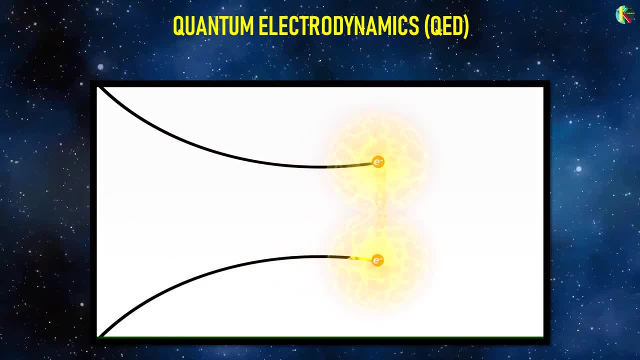 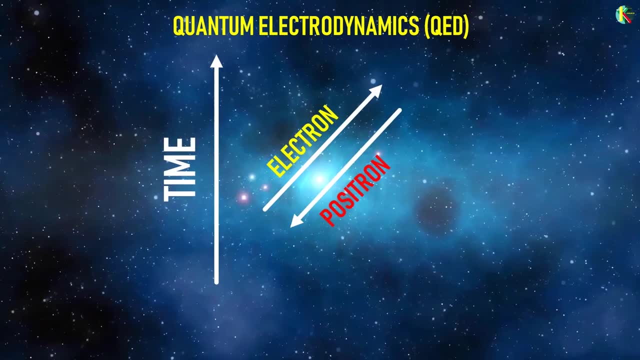 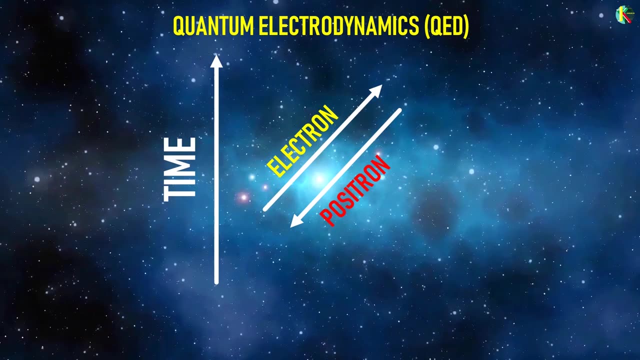 which means interactions between electrons, positrons and photons. In Feynman diagrams we depict the electron as an arrow pointing forward in time or the positron as an arrow backward in time. The antimatter is represented as the time-reversed matter. This interpretation was originally the idea of Ernst Stoeckelberg. The photon 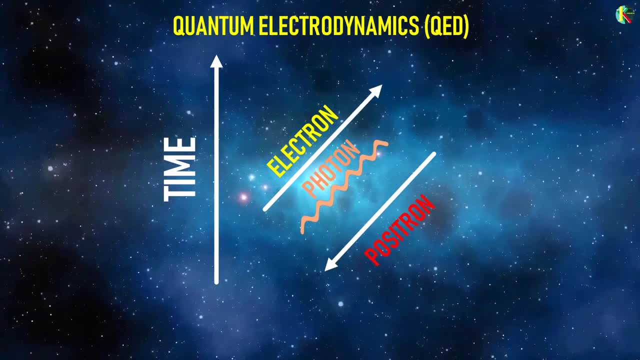 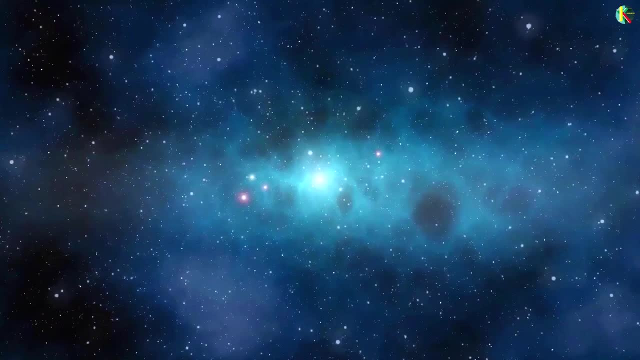 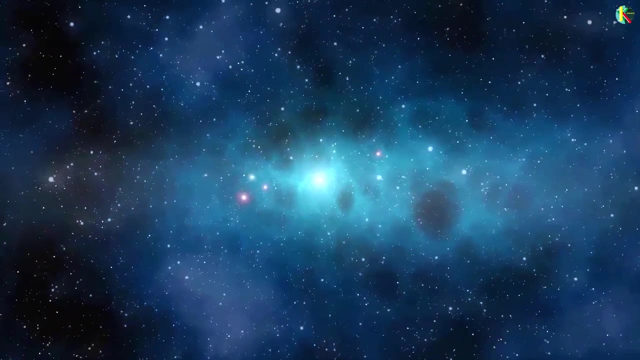 is shown as a wavy line. Time direction is irrelevant for photon. Now the electric and the electromagnetic fields need to interact to give anything measurable. This is where the simplicity nature of this method is seen. Particle or field interactions are represented as a vertex, which is 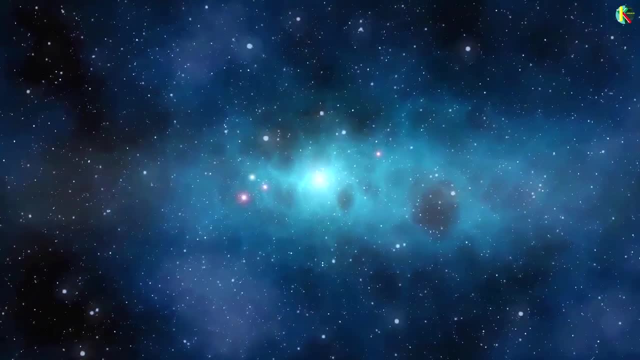 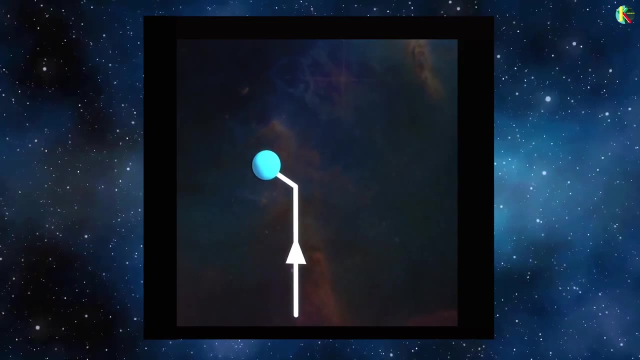 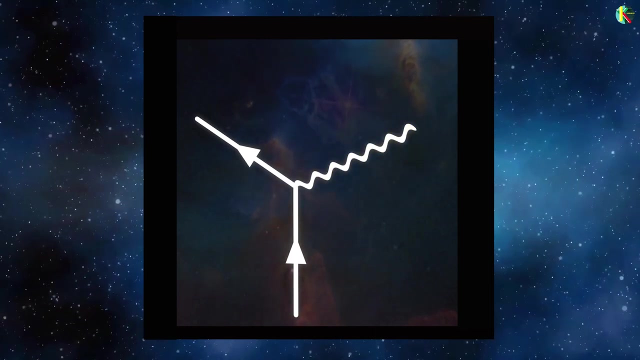 a point where the lines representing the different particles come together. As it turns out that there's only one possible vertex in QED, One with an arrow pointing in, an arrow pointing out and a single photon connection, This vertex alone represents six very different seeming. 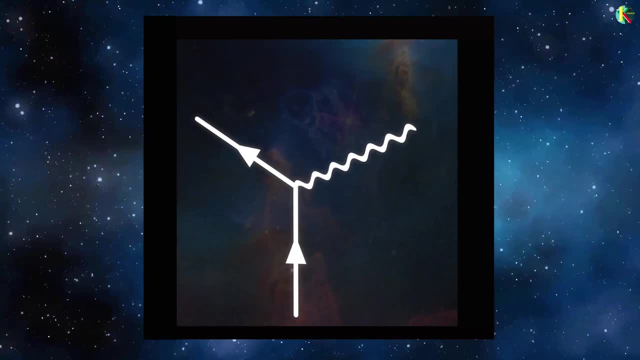 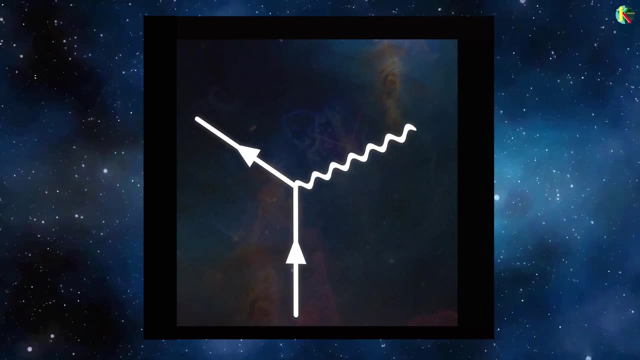 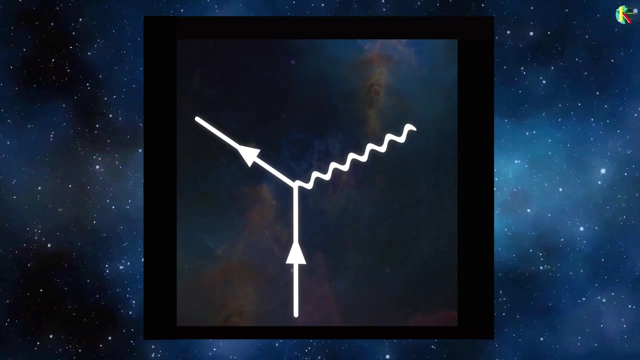 interactions and it can be used to construct infinite Feynman diagrams. Let's have a look at the possibilities. oriented like this, with time increasing upwards. this vertex represents an initial electron that emits a photon, after which both particles move off in opposite directions. but if we rotate this vertex so that photon is coming in from below, we get a picture in. 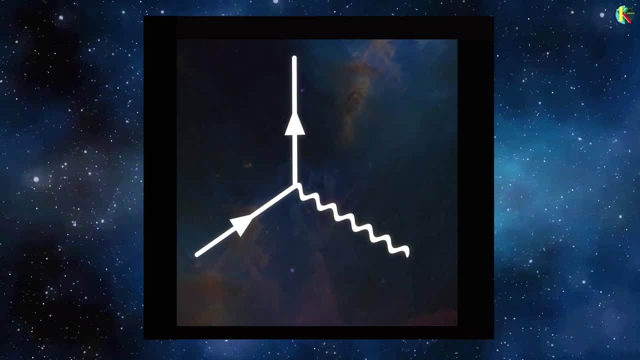 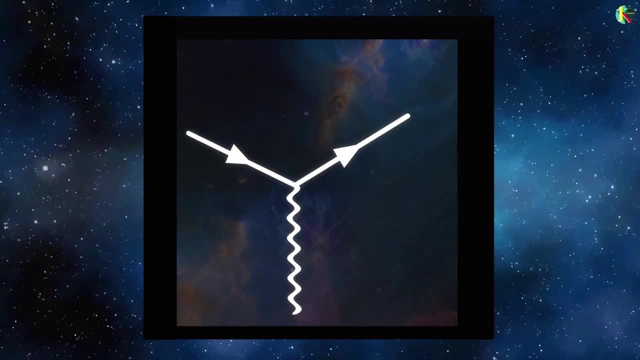 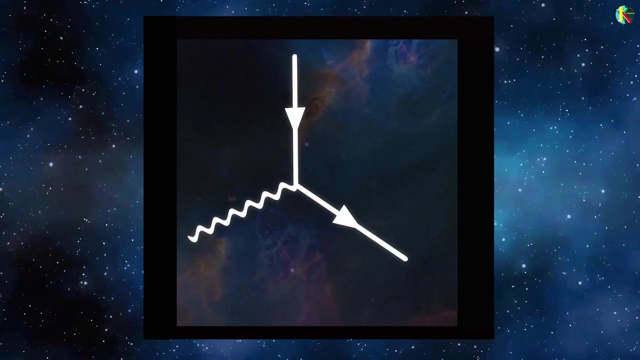 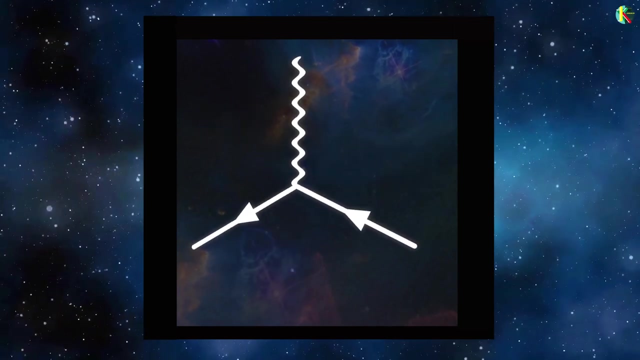 which an electron absorbs that incoming photon. the photon vanishes and transfers the momentum to the electron on rotating again. the picture is a photon coming in and giving up energy to produce an electron positron pair. this is known as pair production. rotate again and now we have a positron absorbing photon and then positron emitting a photon and finally an electron. 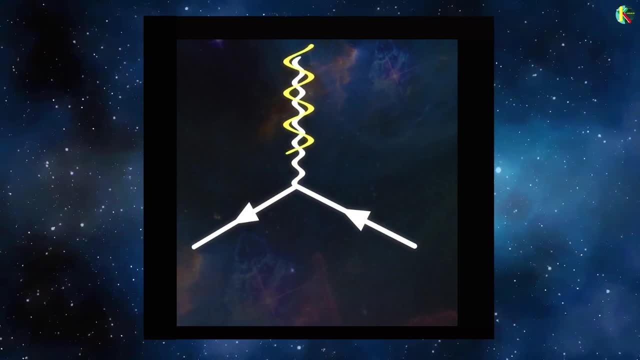 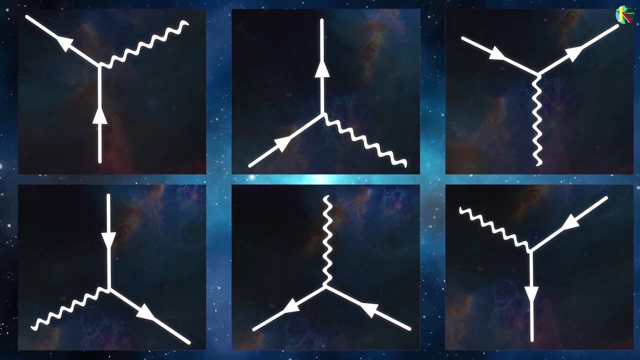 and a positron annihilating each other to produce a photon. this is known as pair annihilation. that's all the ways in which the electromagnetic and electron fields can interact. every single QED interaction is built from these two vectors. The reason is conservation law. Energy and momentum conservation require particles. 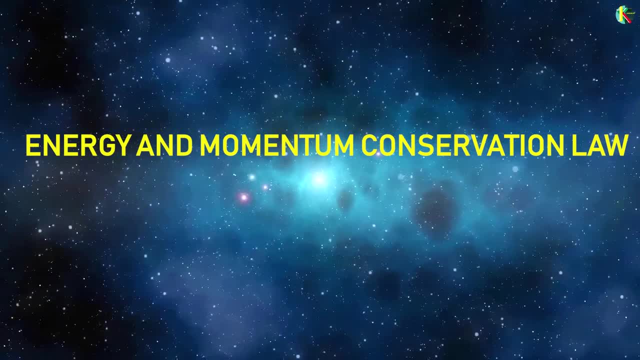 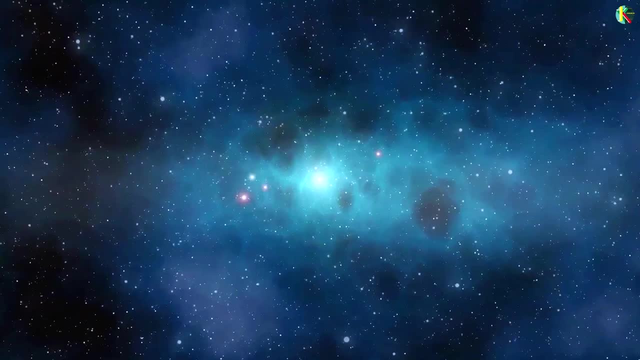 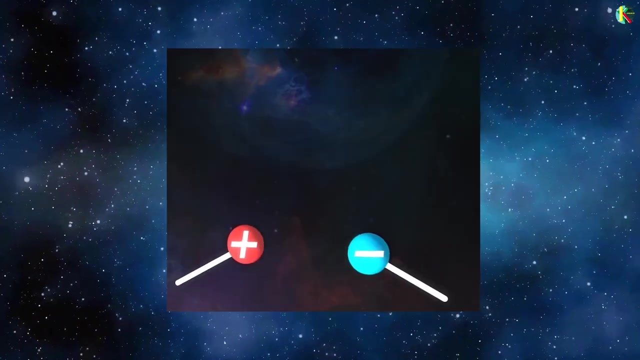 not to vanish or appear from nothing, which guarantees that if something goes in, then something else comes out In addition to that charge must be conserved. If one electron or positron goes in, then one electron or positron respectively must leave. If an electron and 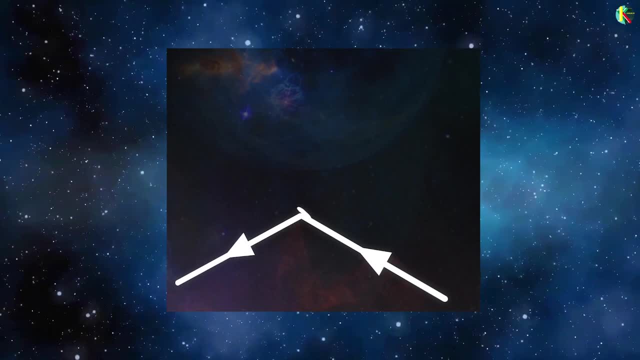 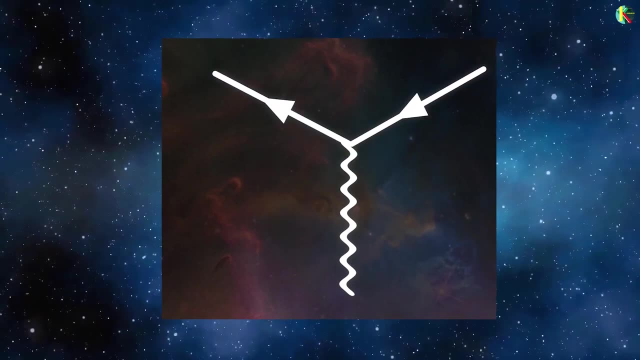 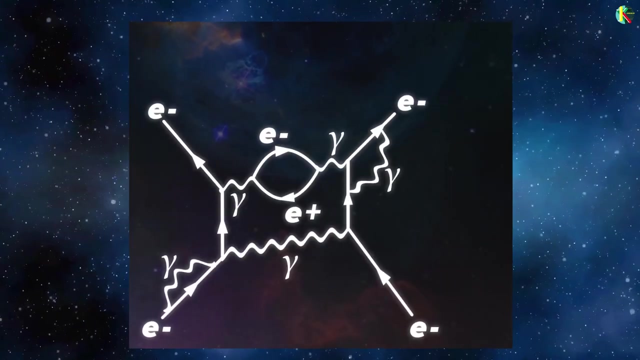 positron both go in, then their charges cancel. so a zero charge photon must leave. Similarly, if a creates a negatively charged electron, it must also create a positively charged positron. There are other, more complex ways in which ingoing and outgoing particles can balance charge. 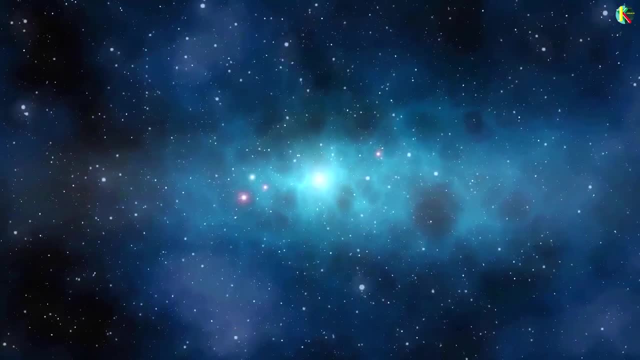 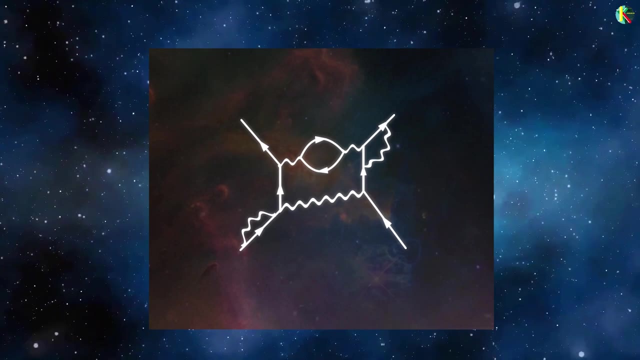 All of these can be built up from this one vertex. Before going any further, we have to know another important rule for Feynman diagrams: The overall interaction described by set of Feynman diagrams is defined by the particles going in and the particles going out. These are the particles we 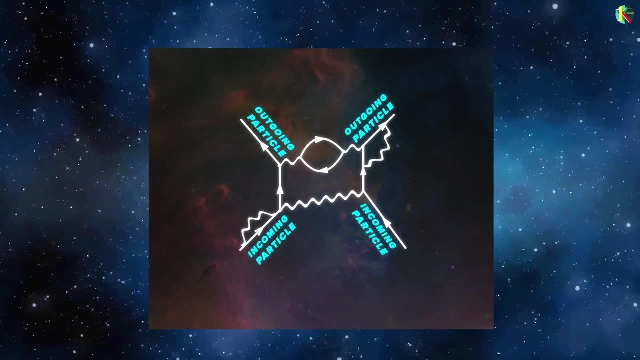 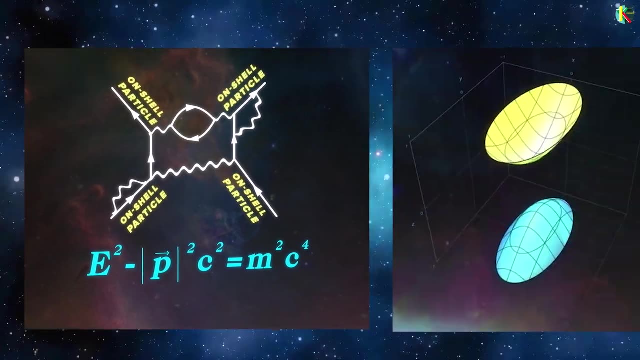 actually measure. The set of Feynman diagrams is defined by the particles going in and the particles going out. These are the particles we actually measure. We know their properties, like energy, momentum and charge. These particles follow Einstein's mass energy equation and are called on-shell particles. They sit on the shell structure we get when we 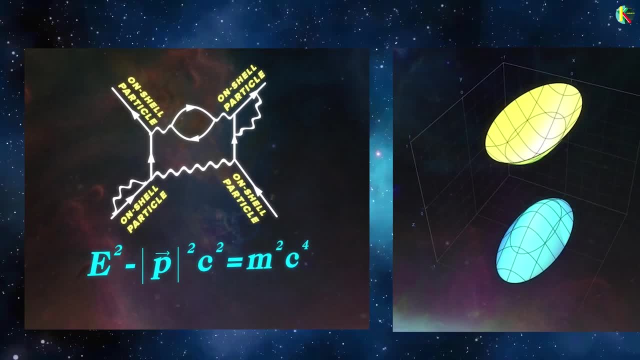 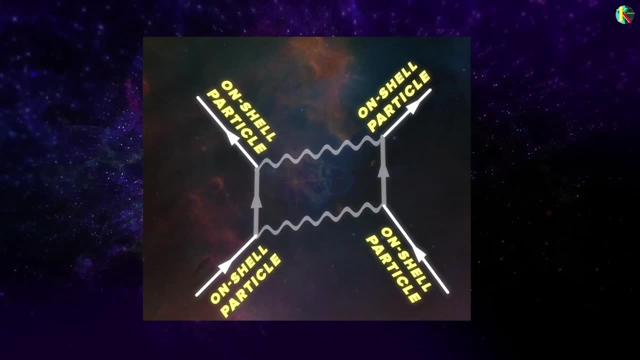 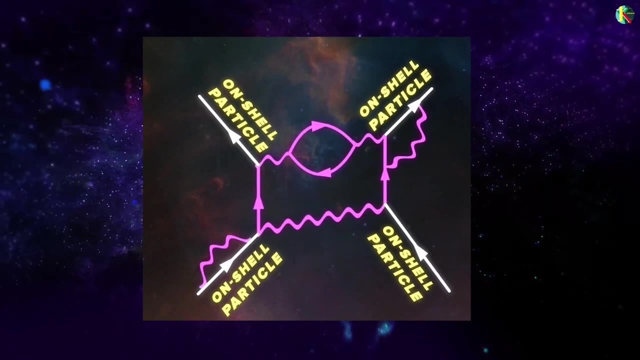 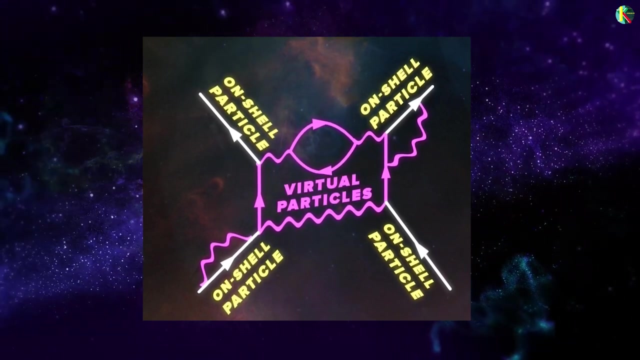 plot Einstein's equation of energy, momentum and mass. On the other hand, everything that happens between ingoing and outgoing tracks has questionable reality. Each possible diagram is a valid part of the possibility space for that interaction. The particles that have their entire existence between vertices within the diagram but don't enter or leave, are called virtual particles. 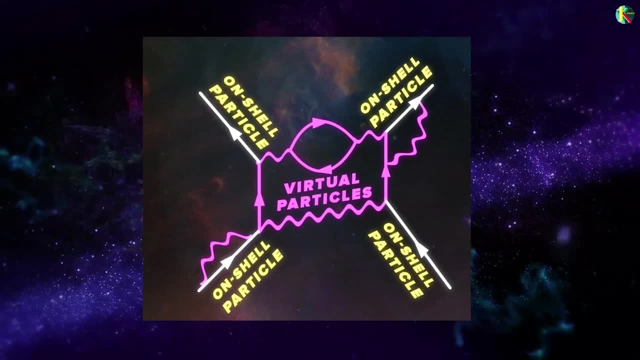 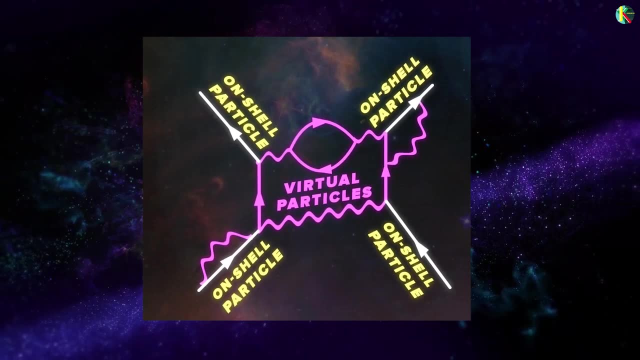 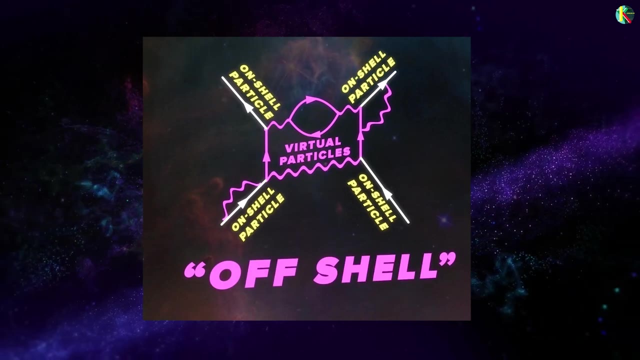 Their correspondence to anything resembling real particles is debatable. They are also, by definition, unmeasurable, Otherwise they would be one of our ingoing or outgoing particles. These particles do not obey mass energy equivalence, so they are called off-shell particles. Electron scattering can be depicted as two electrons going into an interaction and 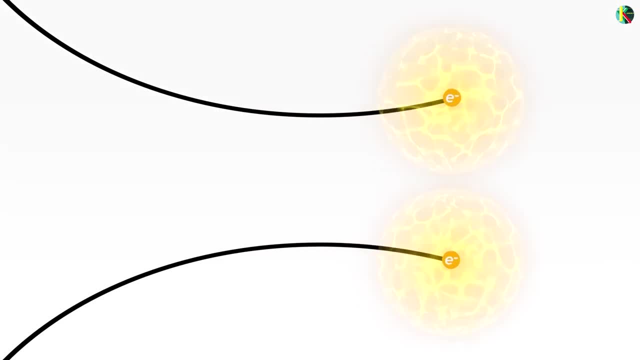 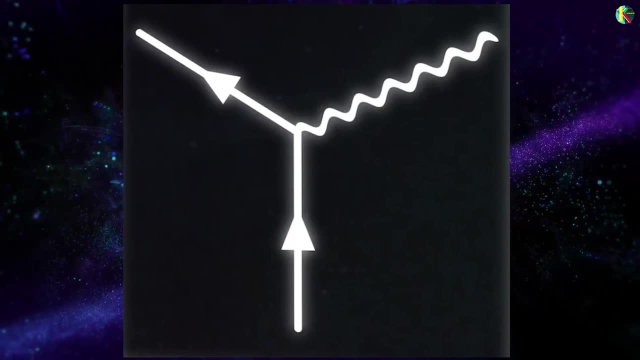 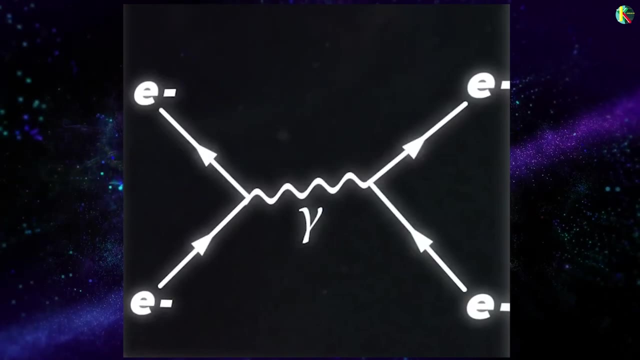 then two electrons going out. We know the momentum of the ingoing and outgoing electrons. Any combination of the fundamental three-path vertex that can lead to this final result has to be considered. Simple examples are the exchange of a single photon to transfer momentum between. 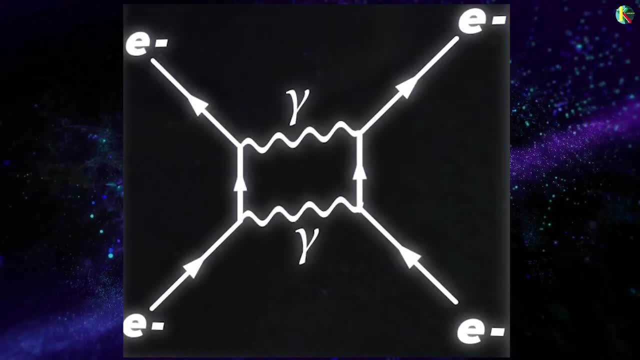 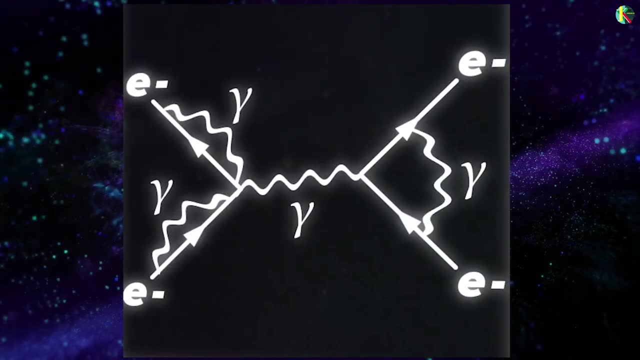 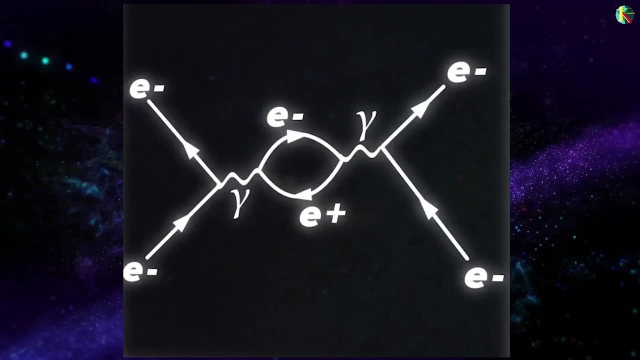 electrons or the exchange of two or more photons, But we can add as many of these vertices as we like, including the electrons exchanging photons with themselves at different stages in the process, Or photons momentarily splitting into virtual electron-positron pairs. Any of these are possible as long as the final result is the same. 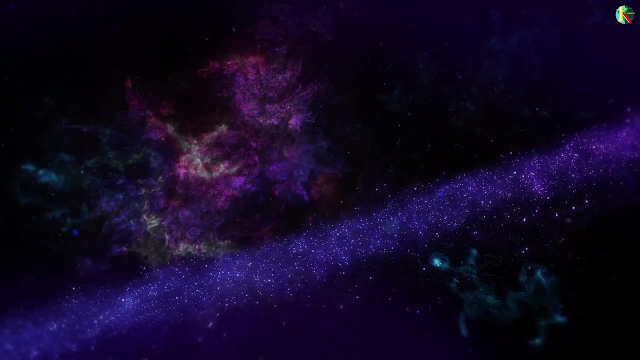 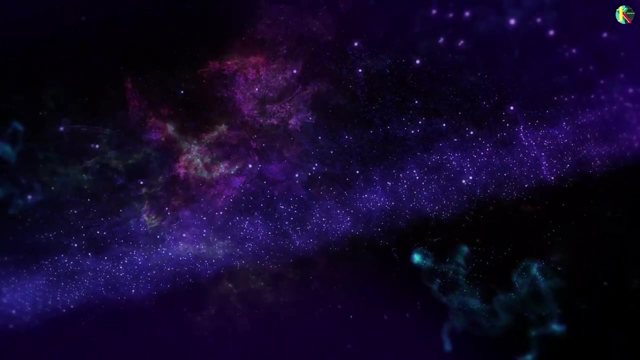 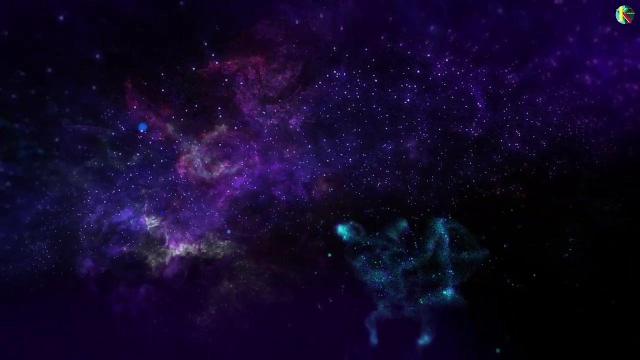 Part of the beauty of Feynman diagrams is that each of these diagrams themselves represents an infinite number of specific interactions. Each of the particle paths are actually infinite paths, as well as infinite possibilities for particle momentum. We have to consider even impossible faster-than-light paths for any particle. 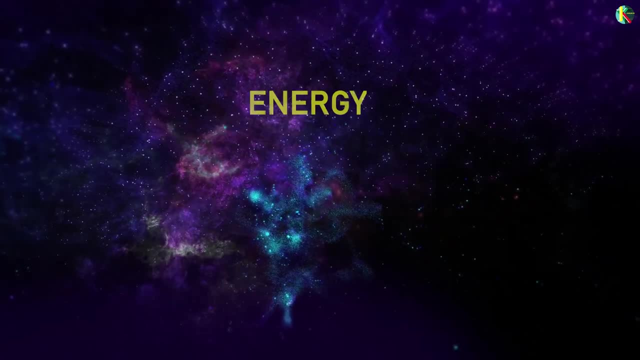 besides the ingoing and outgoing electron-positron-positron-positron-positron-positron-positron-positron-positron-positron-positron-positron. The last point is really powerful For two electrons exchanging a single photon. 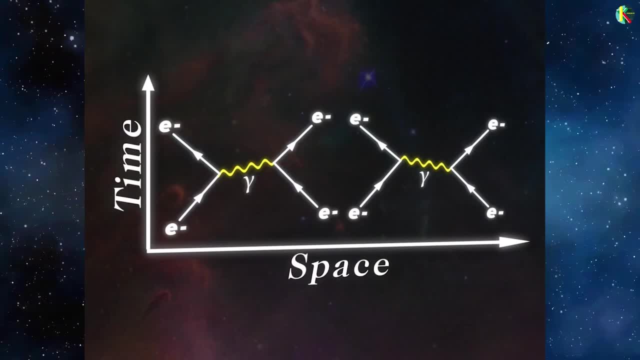 it doesn't matter if we draw the photon going from the first to the second, Even though this seems like a very different interaction. we can think of the differences just being the photon travelling forward in time in one case and backwards in the other. The math didn't tell us how precise the interaction was. 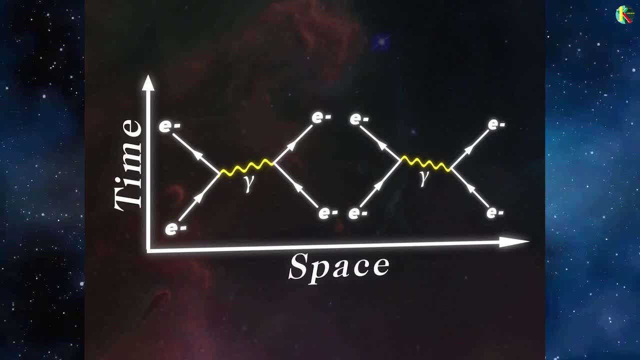 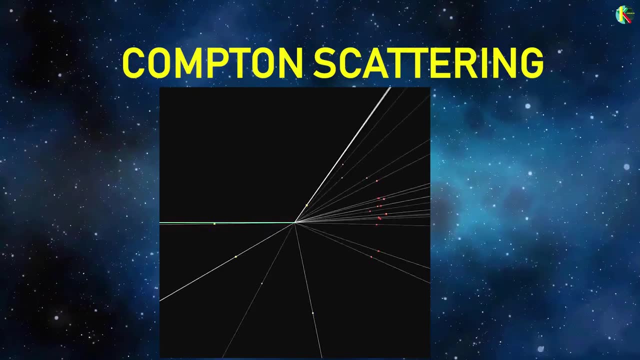 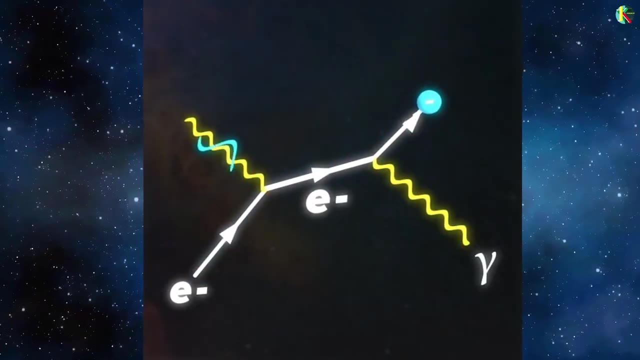 case and backwards in the other. The math describing the transfer covers both cases. Let's look at another example of Compton scattering. In this process, an incoming electron and an incoming photon bounce off each other. One way that can happen is for the electron to 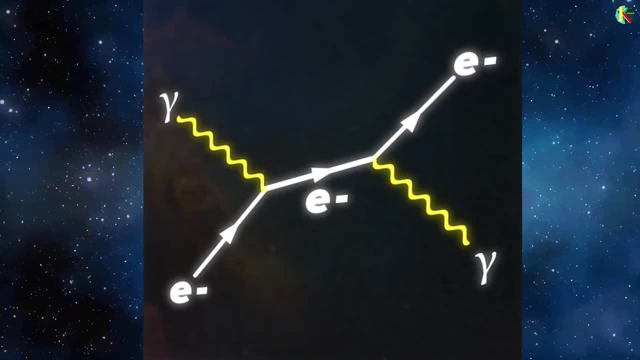 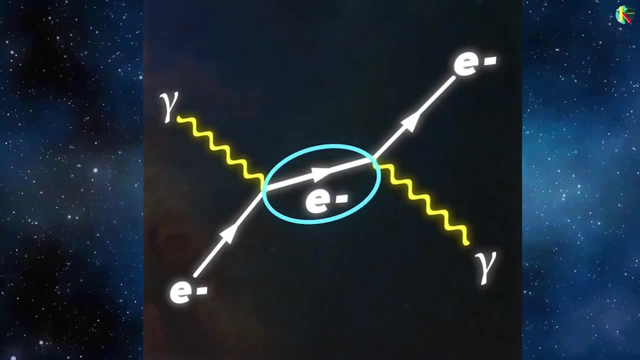 emit a new photon and later absorb the old incoming photon. In that intermediate stage between vertices the electron is a virtual particle, which means we include all possible paths it might take, as long as they lead to producing the same final electron and photon. 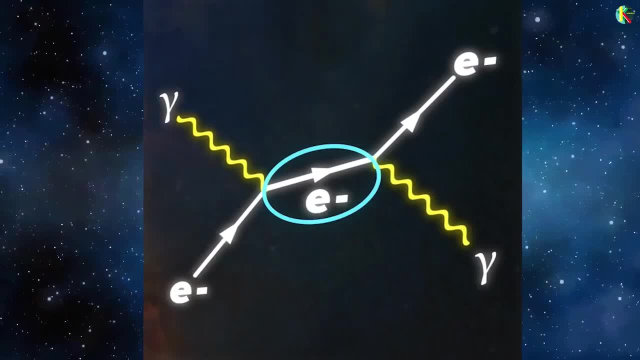 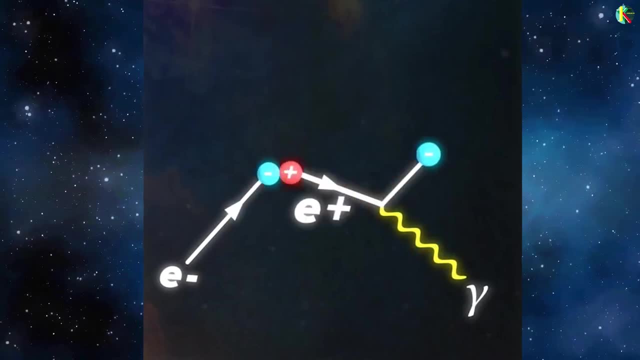 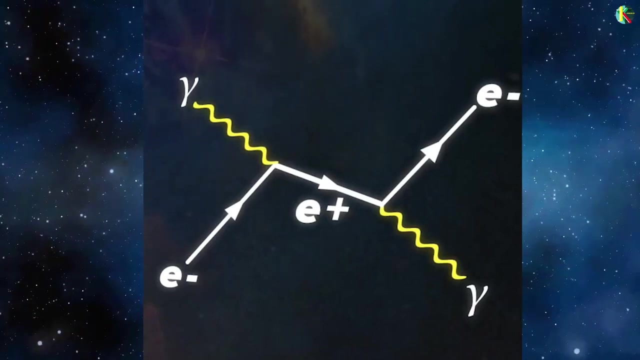 That also includes paths backwards in time. Mathematically, a time-reversed electron looks exactly like a positron. Like in this situation, the same particles go in and out, But now the interactions look very different. Instead of an electron emitting and then absorbing a photon, 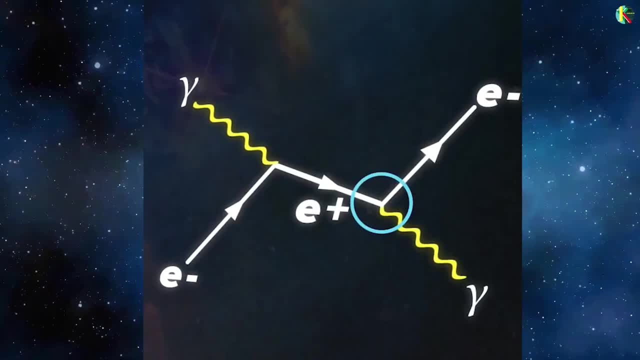 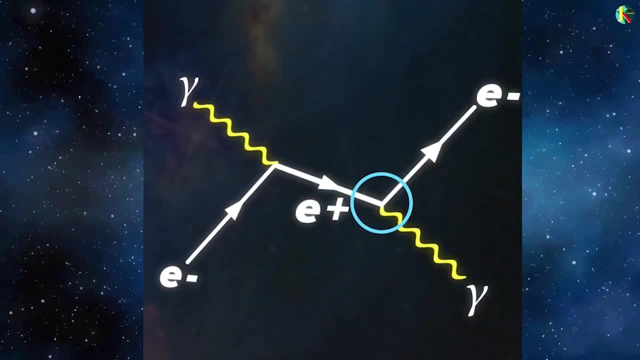 we have on one side that incoming photon creating an electron-positron pair, that new electron-positron pair and that new electron-positron pair, The positron, becomes our outgoing electron. but the positron annihilates with the incoming electron and produces the outgoing photon. These may seem like widely different processes. 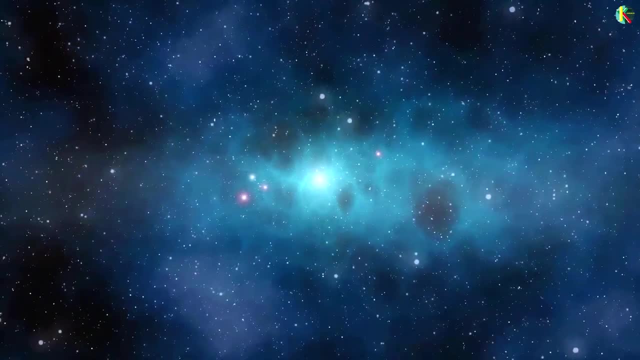 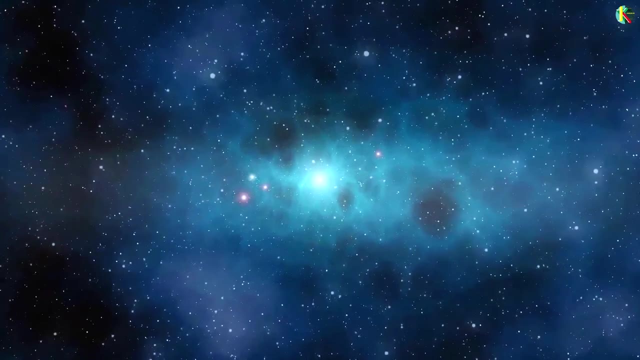 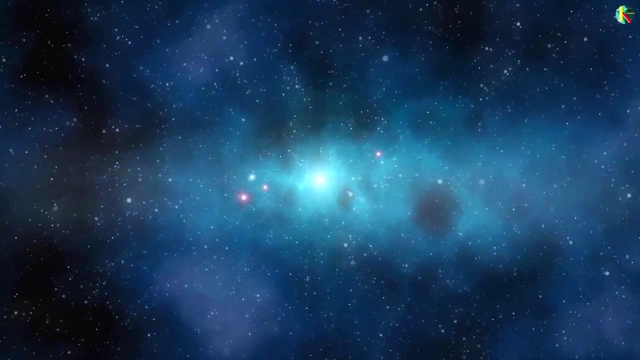 but in the math represented by Feynman diagrams, they are exactly the same. The interpretation of the interactions is irrelevant. All we care about is the topology of the diagram. In other words, how are the vertices connected to each other? This fact makes Feynman diagrams